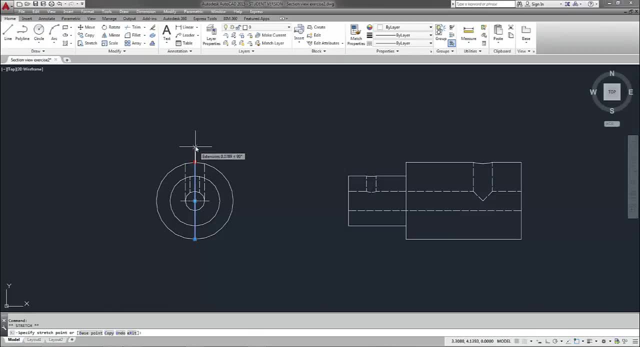 And I'm going to select this line. so I have some grips that will allow me to extend my line straight up And I'm going to use my ortho one, so it's going to constrain my movement vertically and horizontally. So I want to extend the end points of my line segment just beyond my part here. 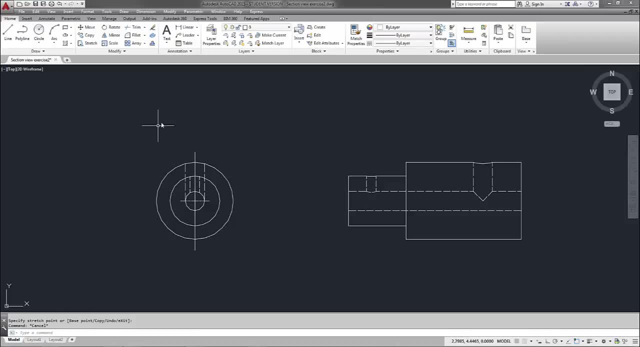 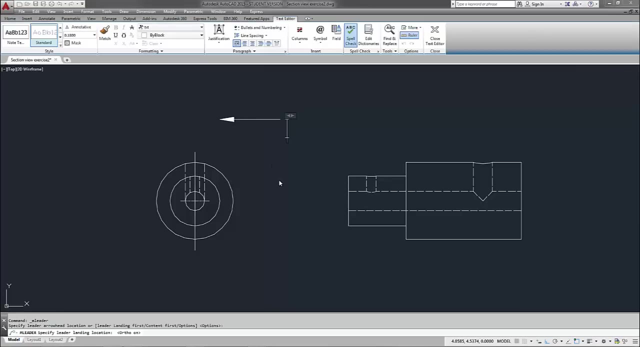 Now I want to add my arrows that determine my line of sight, And I do this by going to the leader command and placing a leader anywhere in the drawing. Now I turn ortho one And as soon as it prompts me to enter a text, I'm going to leave the text out. 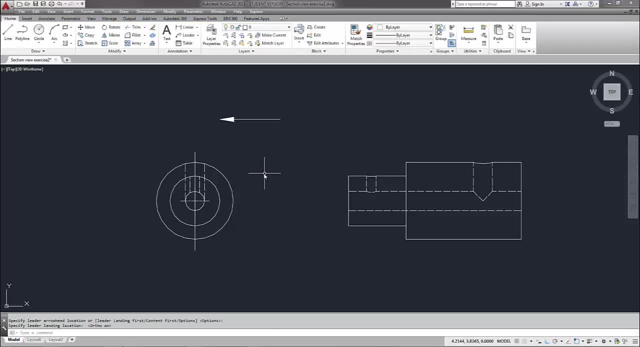 So I'm just going to click somewhere in my graphics window here And I'm going to need to explode this leader, And when I do that I'm left with an arrow and two line segments. This is actually the landing of my leader here. 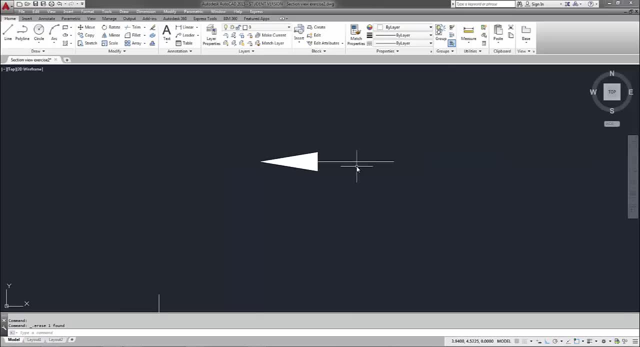 So I'm just going to select that and then delete it. So I'm left with an arrowhead and one line. Now I can use my move command along with my snap To snap the end point of the arrowhead onto the end point of my line. 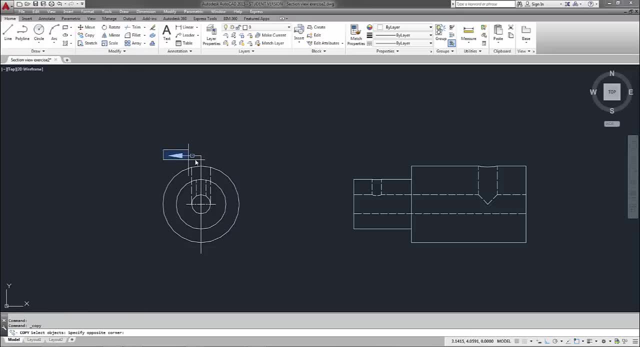 Then I can use my copy command to copy this straight down from the top of my line segment to the bottom, And there is my cutting plane line. It cuts right through the middle of my part. Now there's one more thing I need to do. 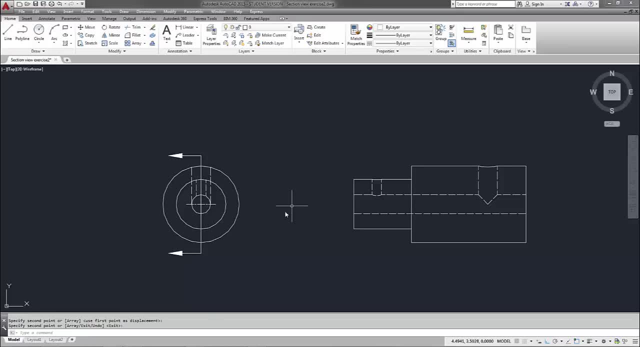 I need to convert my line type here on my cutting plane line to phantom line type. Now, a lot of people get in the habit of changing their properties Right here in this section of the ribbon. I try to avoid that And I try to let my layers dictate my line types and my line weights. 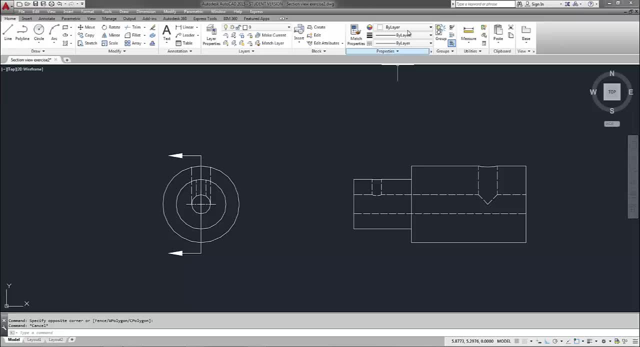 As well as my colors, whenever possible, And I will come up here on occasion and use this to change very specific properties of one or two entities. So I'm going to come up to my layer properties manager And I'm going to create a new layer. 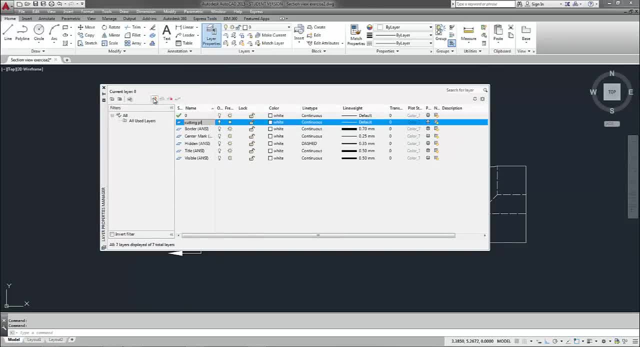 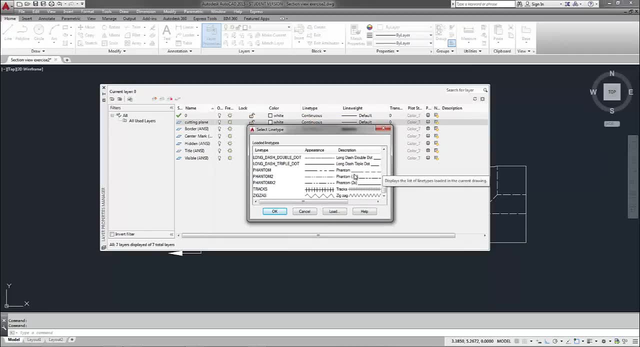 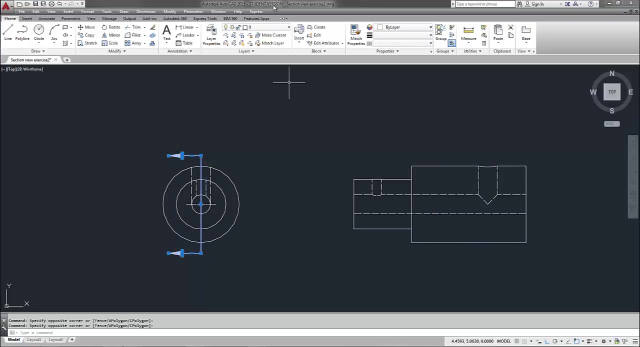 And I will call this cutting plane And I will change my line type from continuous To phantom, Alright, And I'm not going to worry about line weights right now. So I'm going to select my cutting plane, line Arrows and lines. 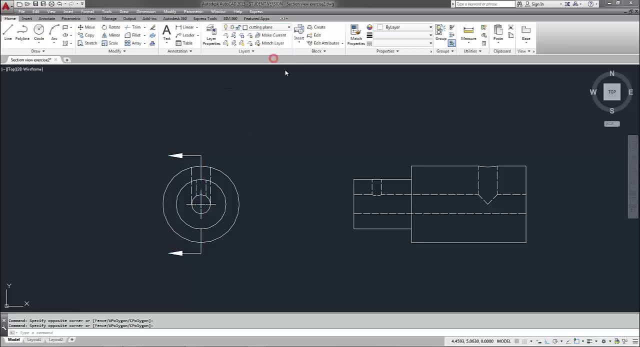 And I will select the cutting plane layer to move it over. There it is So with my center mark here. It's not quite clear what I've got going on with my cutting plane line. It doesn't really accurately look like a phantom line type. 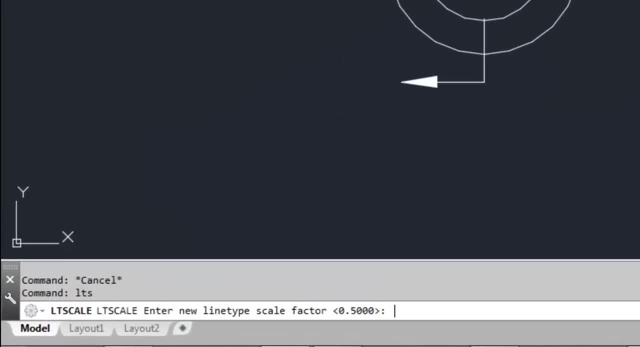 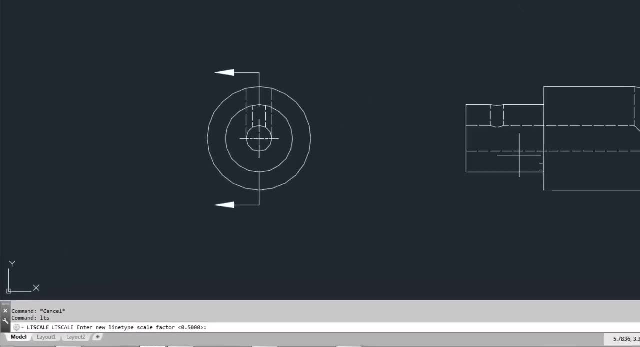 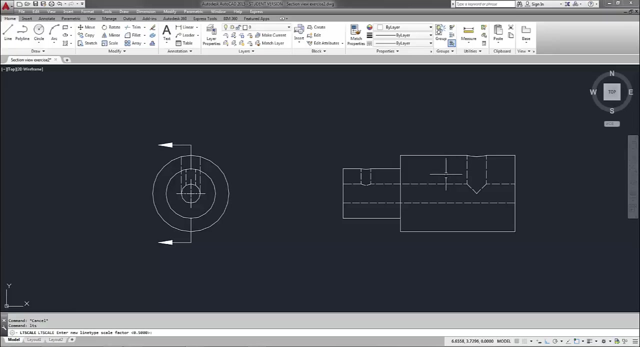 So I can adjust my line type scale. I can key in LTS And currently I've got it set at .5.. And I have it set at .5 because that's what I have decided looks good or acceptable for my hidden lines. So I don't really want to change my global scale factor here. 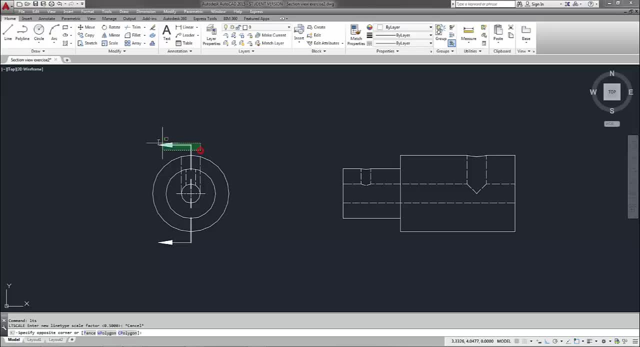 But I still want my phantom line to look As it should. So I'm going to select these And I am going to do a properties change just on the items that I have selected. So I'm going to come up to my properties. area of my ribbon. 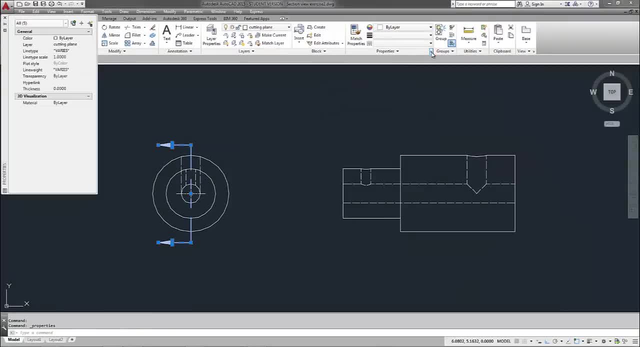 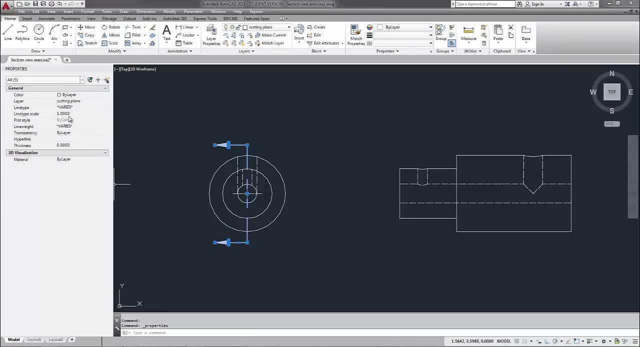 And I'm going to click on this little diagonal arrow here And that will bring up my properties dialog box. Now, the properties box here. I'm going to go ahead and dock it on the left hand side. It gives me all the information. 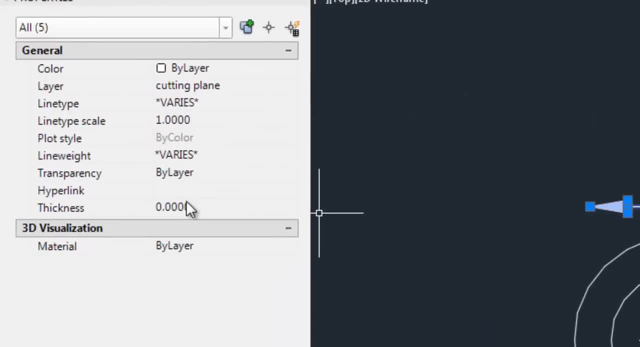 All the properties for whatever I currently have selected. So the line type scale Right now is at 1.. Now this is different from the global scale. If you remember, the global scale when I keyed in LTS was at .5.. Now this line type scale is relative. 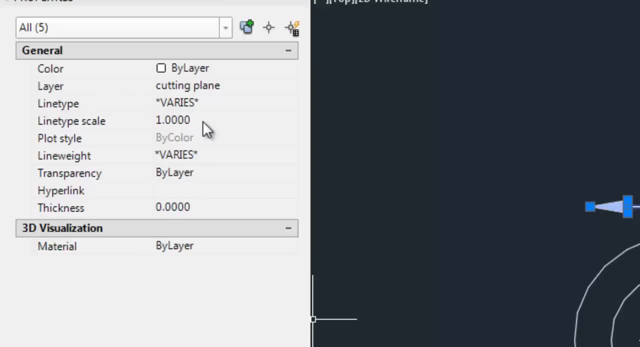 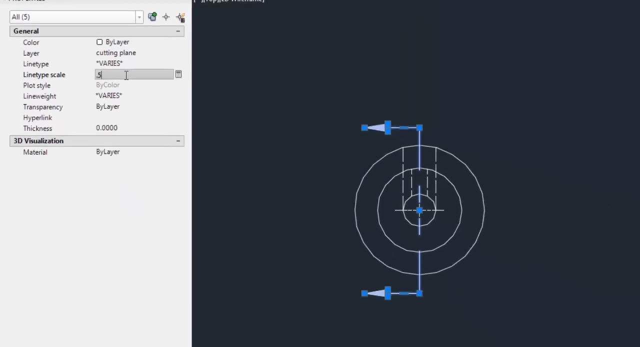 So it's telling me that it is a line type scale of 1 relative to my global scale of .5.. So what I'm going to do is change this right here to .5.. And that is actually half or .5 of my global scale. 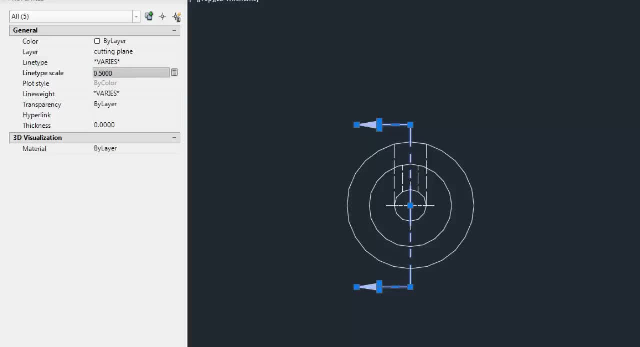 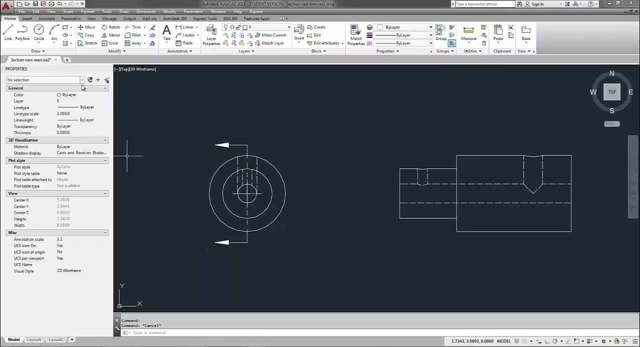 So this .5 is half of my global scale. So in other words, it's truly a line type scale of .25.. Now, graphically this looks a little bit closer to what I need for my cutting plane line. So I'm just going to close out that properties box. 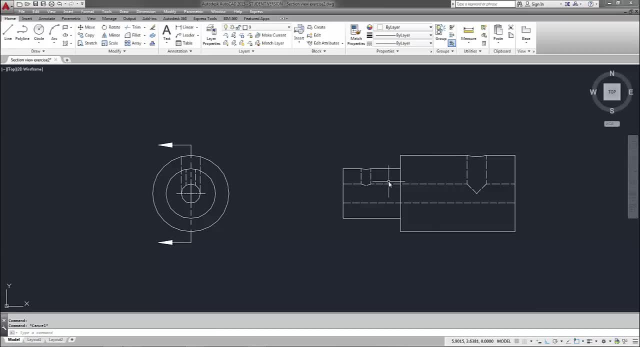 Now I'm ready to come over to my right side view and convert this to a section view. So basically, what's going to happen here is all my lines that are hidden in a proper section view will show as object lines. So I'm just going to simply highlight all of my hidden lines. 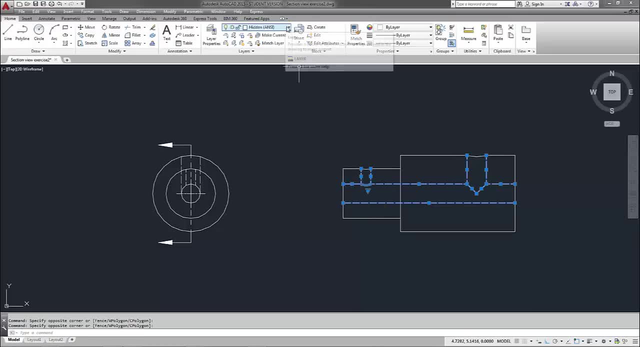 All of my hidden entities here And I'm going to move them onto the visible layer And notice they're all solid lines now because I have my line type set up in my visible layer as continuous line type. I'm also going to need to trim out this edge here because that's not going to show up inside the parts. 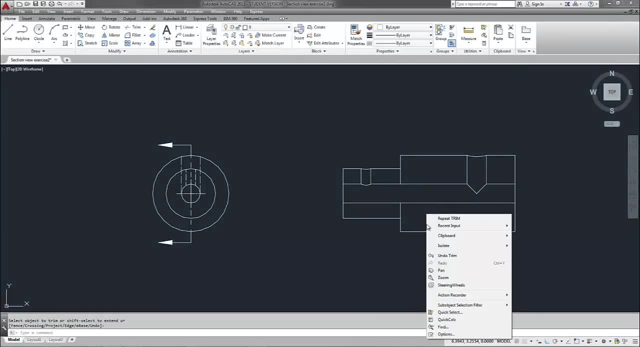 Alright, Now actually, I'm going to have to do the same thing on here as well. There we are. Now I need to add my hatch lines. The hatch lines represent the solid material of my part. So if I'm actually cutting through material, I need to represent that by using my hatch lines and showing the section lines of certain areas of my view here. 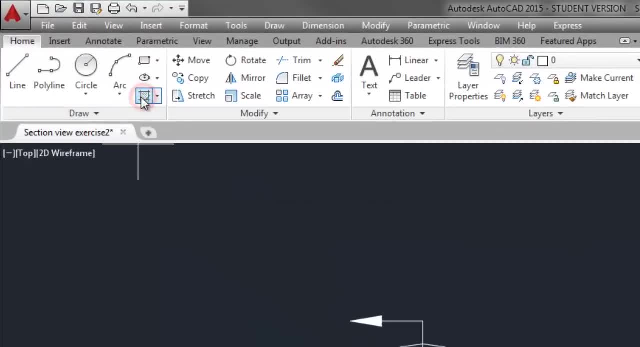 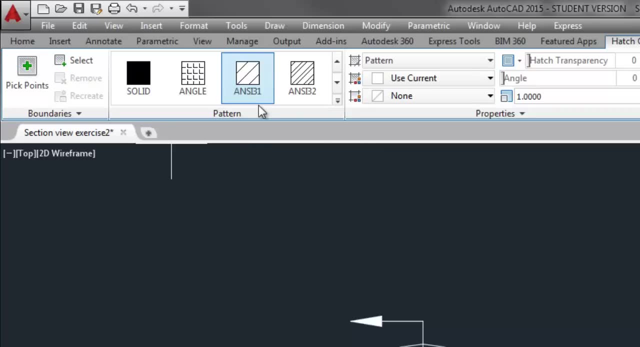 So I'm going to come up to the draw section of my ribbon and select hatch, And when I do that, my ribbon will convert to all of my hatch lines And, by default, AutoCAD automatically selects ANSI 31.. Which is good, because that's what I'm going to use. 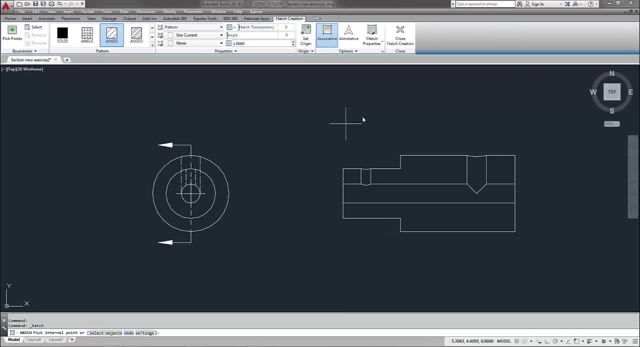 ANSI 31 represents just general material, so I can kind of use it for anything. It works for this part because I have yet to actually select a material. So if I just move my crosshairs down to a certain section, it'll show me a preview of what those section lines will look like. 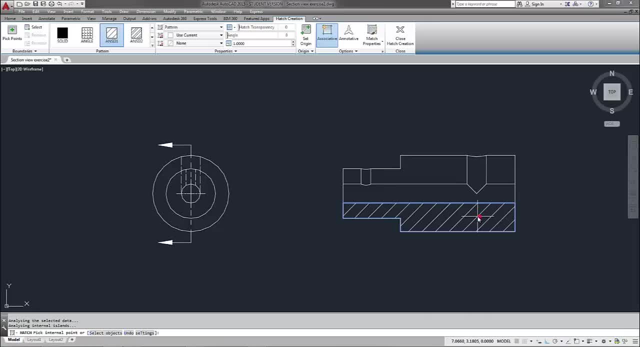 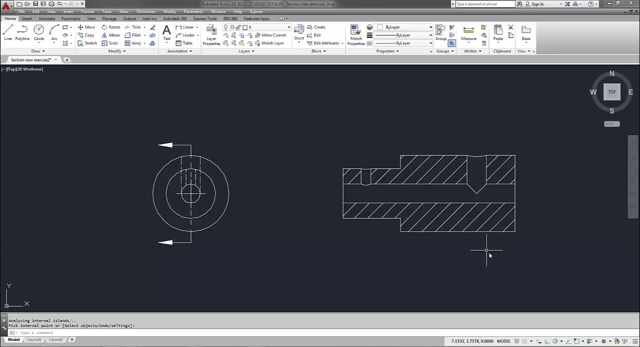 And if I like what I see, I'm just going to click. So I want my section lines here. Don't need it there. That's actually a hole. This is also a hole. I do need it here and here, Alright. So all those hatched areas represent solid material that I'm cutting through to show my section view. 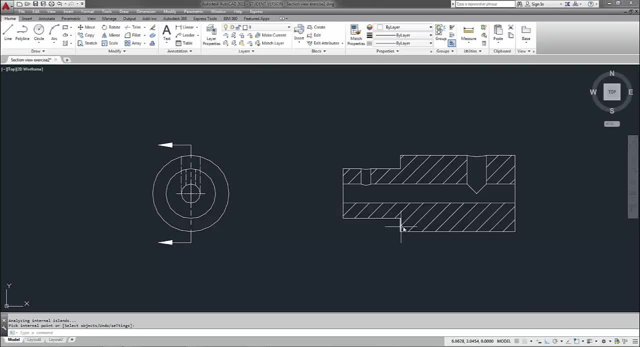 What we're actually seeing here with the other lines are the edges that exist as part of the internal holes. We are actually looking directly at the inner surface of those holes, So we're not going to hatch that part. Now. if I want to change the scale of the hatch, I'm not going to do it through my LTS or my line type scale command.